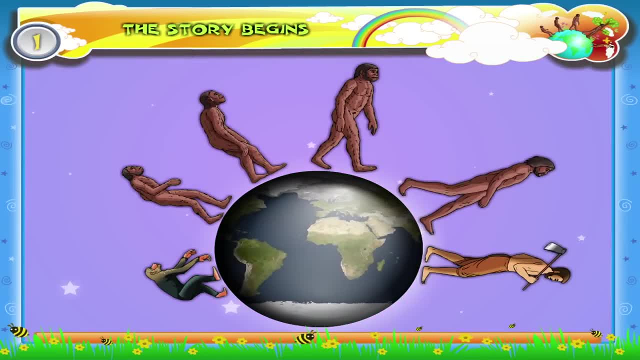 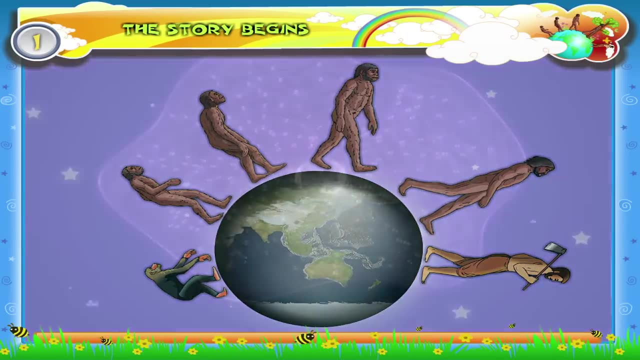 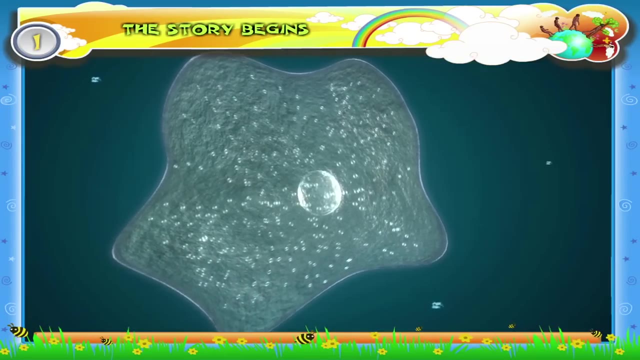 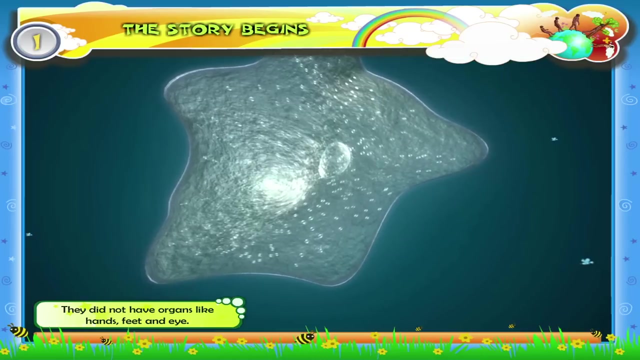 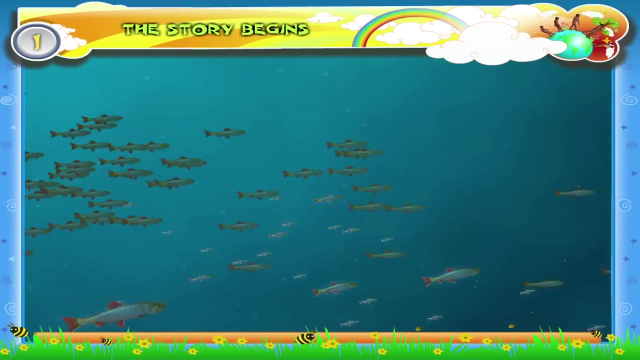 One such evolution worth mentioning is that of man. The story of evolution begins quite interestingly. The first living things were born in water. They were so tiny that they could hardly be seen. They did not have organs. They had hands, feet and eyes. Then many years passed and there appeared animals that could live on land and water. 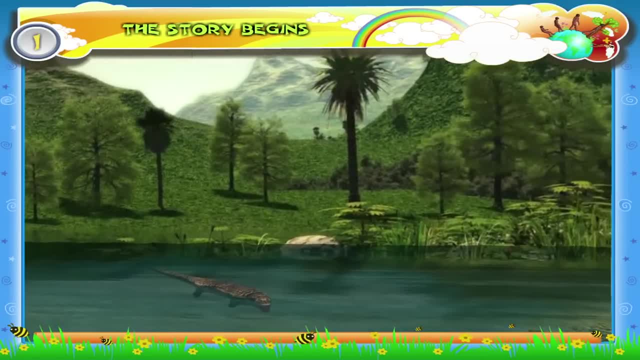 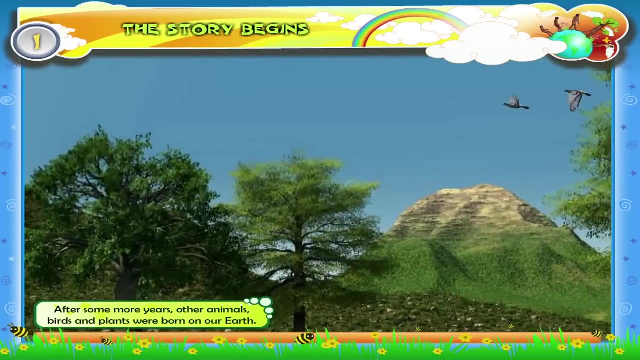 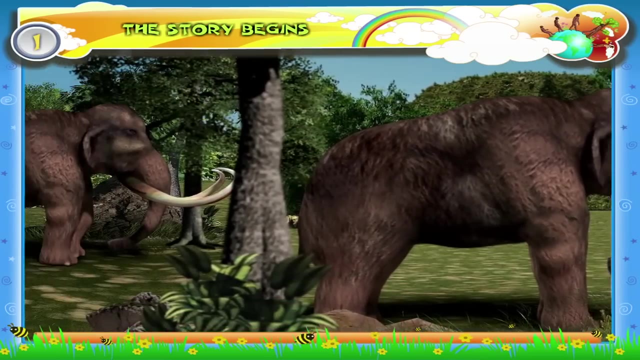 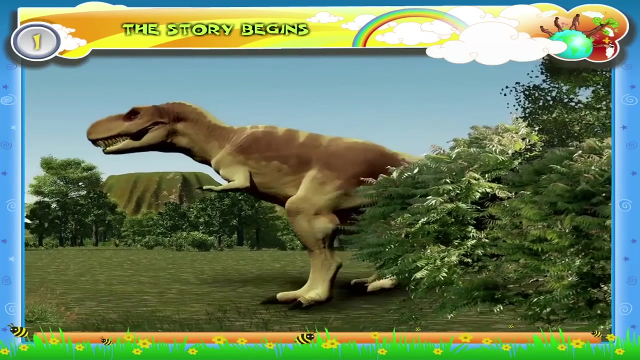 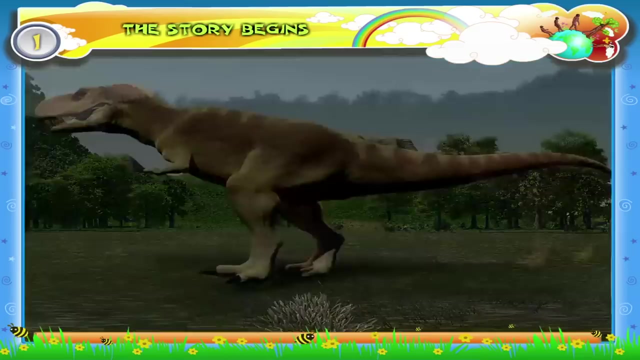 Some such animals were the frog, the crocodile and the tortoise. After some more years, other animals, birds and plants were born on earth. Some animals were even larger than elephants. Gradually, these large animals became extinct. They all died and disappeared completely from the earth. 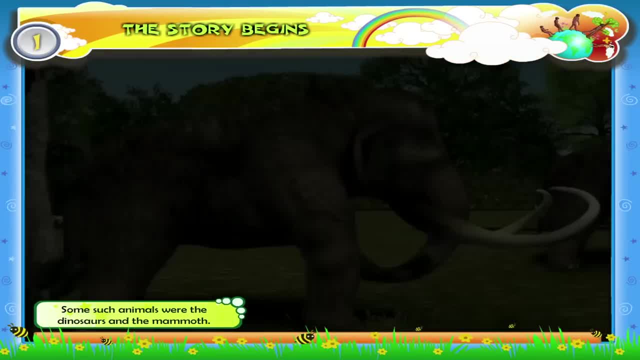 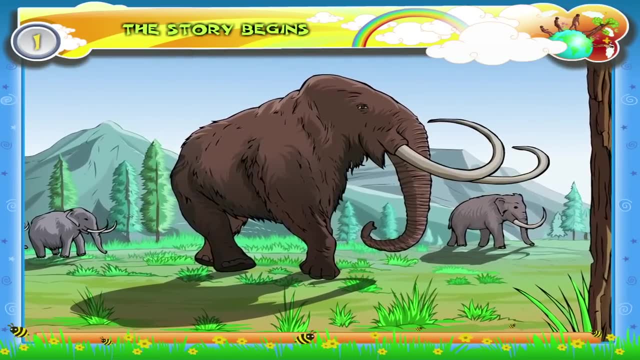 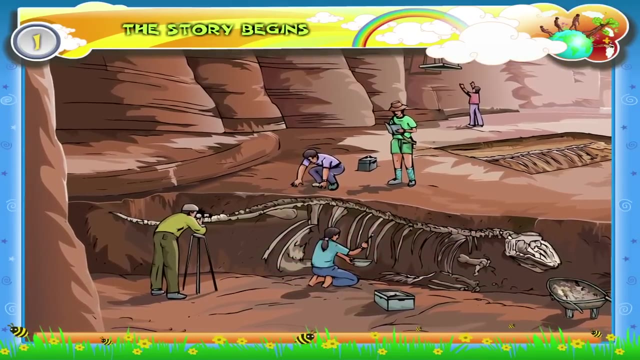 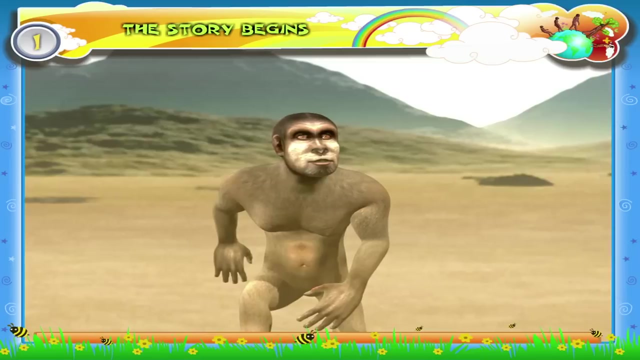 Some such animals were the dinosaurs and the mammoth. Hmm, you may wonder how we know so much about these large animals. Well, their skeletons have been discovered deep under the ground. Many years after the dinosaurs became extinct, a monkey-like creature was born. 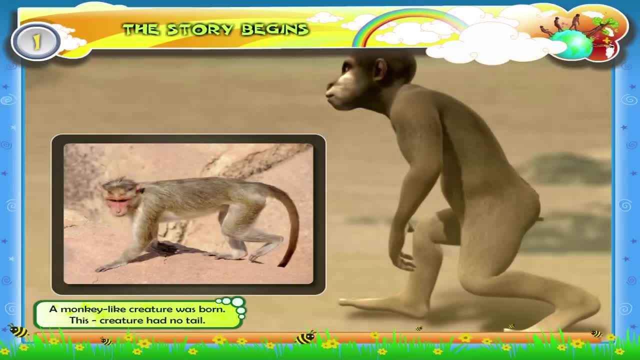 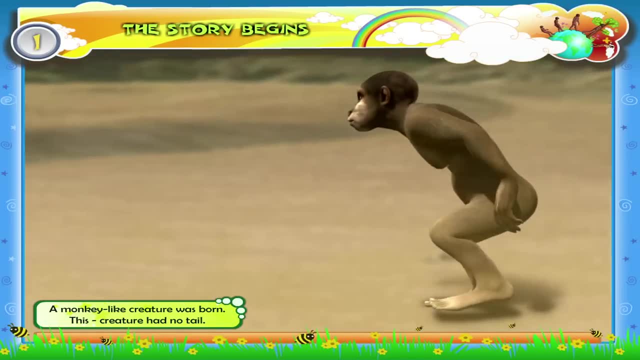 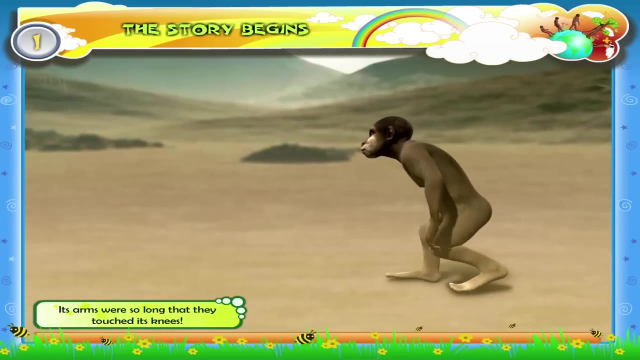 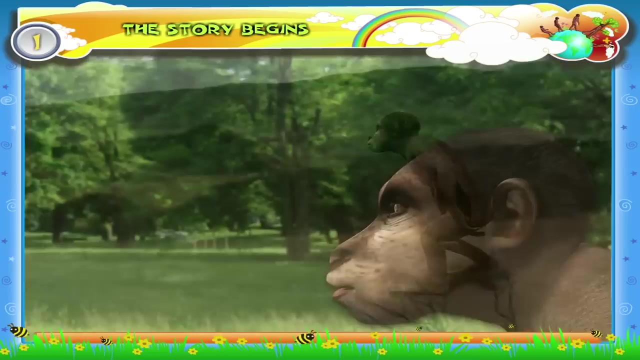 This creature had no tail. Well, its head was bigger than that of a monkey. It could walk on two legs, but could not stand or walk erect. Its arms were so long that they touched its knees, And it was hairy too. Have a close look at the face of this creature. 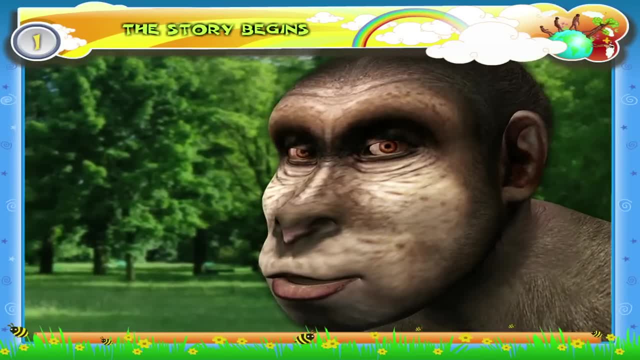 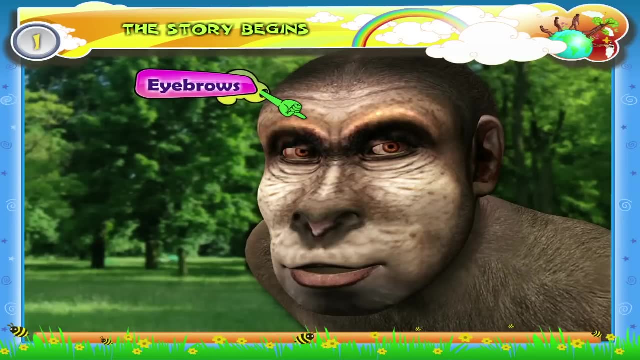 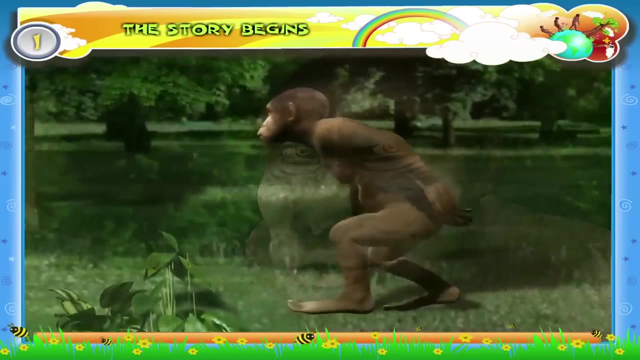 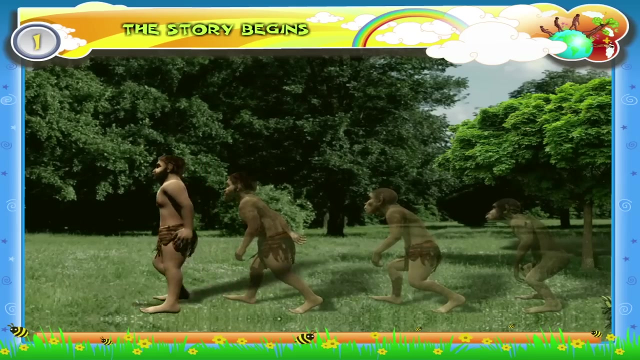 Hmm, don't you see something different? Yes, He looks different from all of us. His eyebrows were thick, his nose was flat and his jaws were broad. After many years, the bodily features of this monkey-like creature changed gradually. He could walk straight. 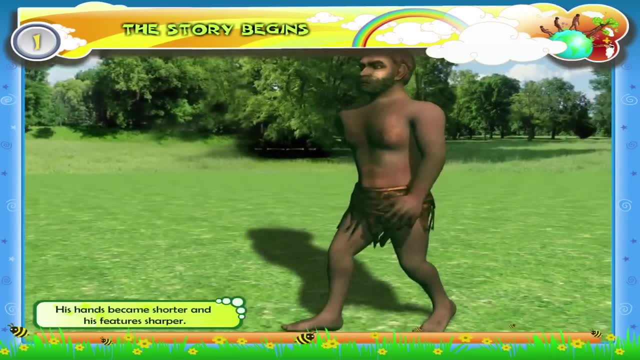 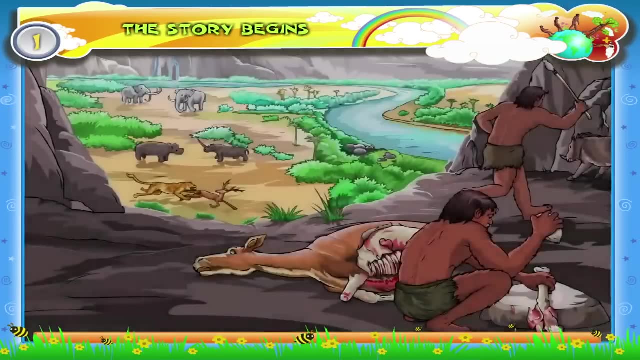 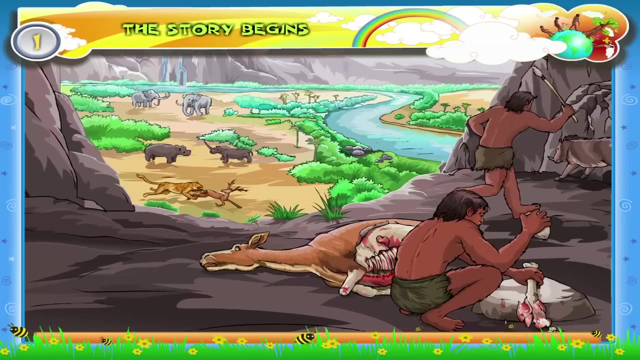 His hands became shorter and his features sharper. He began to look like a man. It was like he was walking with his own hands. He was not the same man we see today. People like to call him a man because he is not the same as the man we see today. 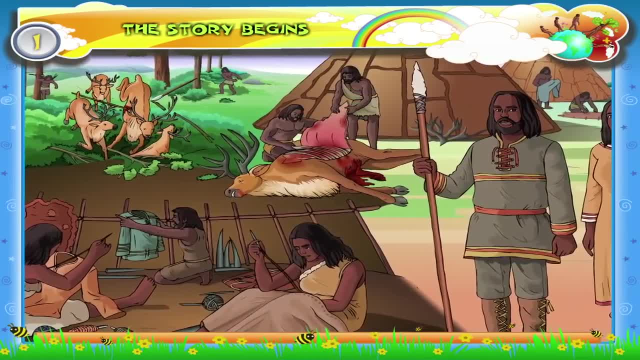 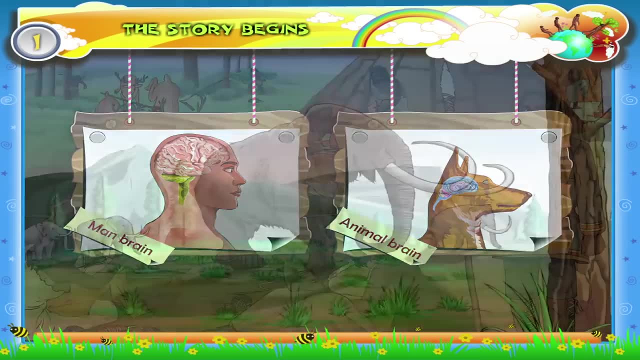 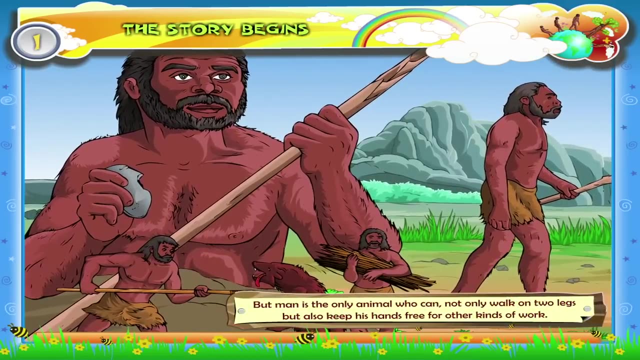 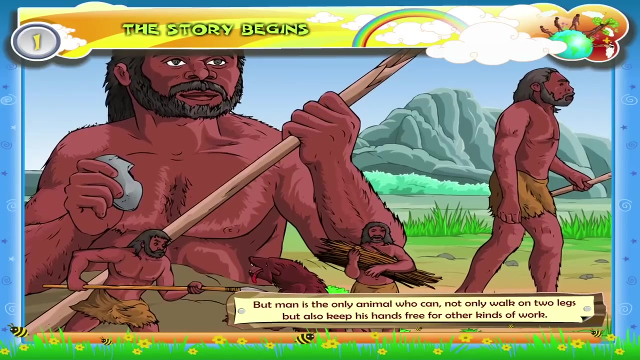 Man too is an animal. He lived on Earth with the other animals, But he was different from all of them. Man is the most intelligent of all the animals, But man is the only animal who can not only walk on two legs but also keep his hands free for other kinds of work. 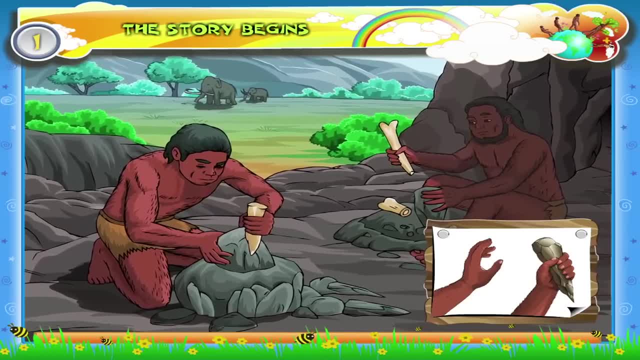 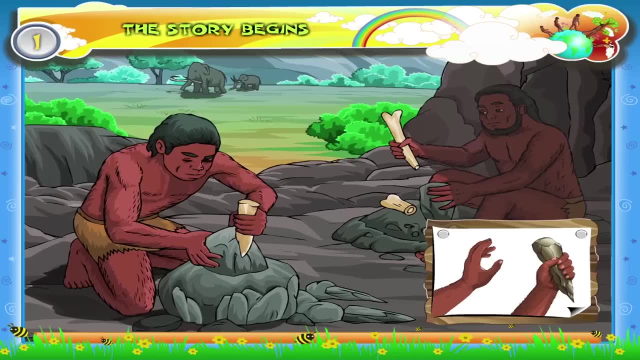 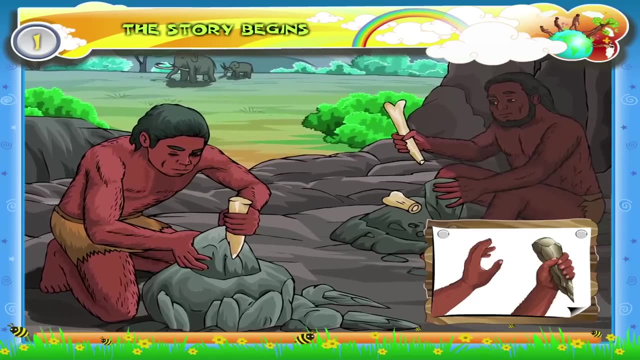 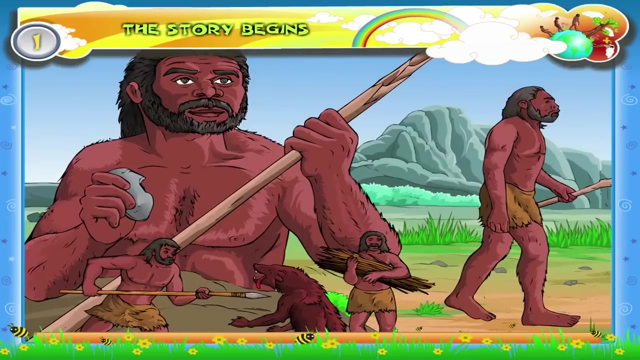 Now look at this picture. Man can move his thumb and bring it in front of the other fingers. He can hold things easily. He can also make new things with his hands. Try it, You can also do the same. There is something interesting you must know about man. 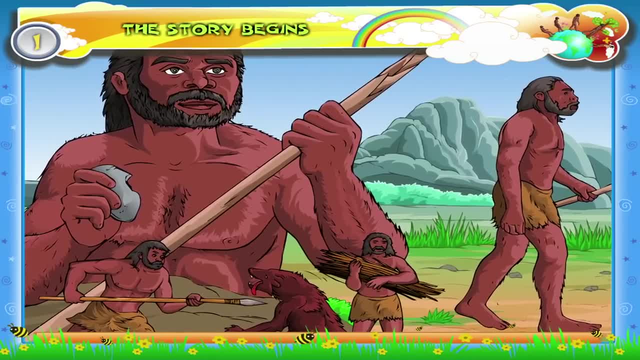 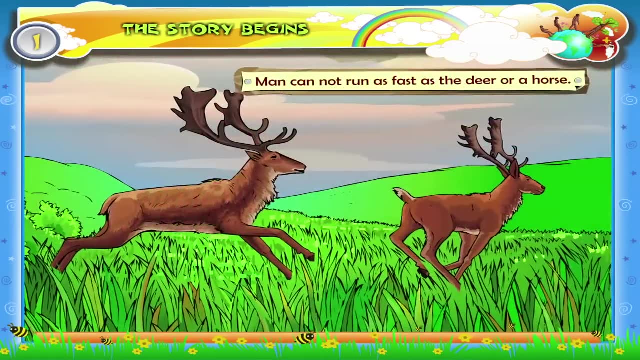 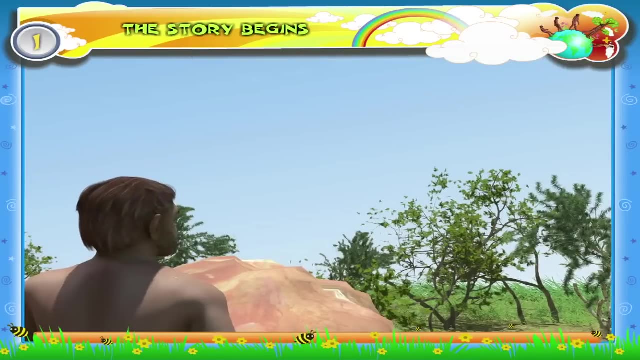 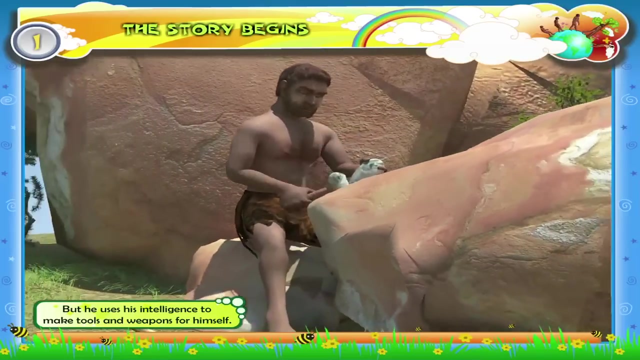 Although he is the most intelligent animal, he is not stronger than an elephant or a tiger. Man cannot run as fast as the deer Or a horse. Man can also not fly like the birds, But he uses his intelligence to make tools and weapons for himself. 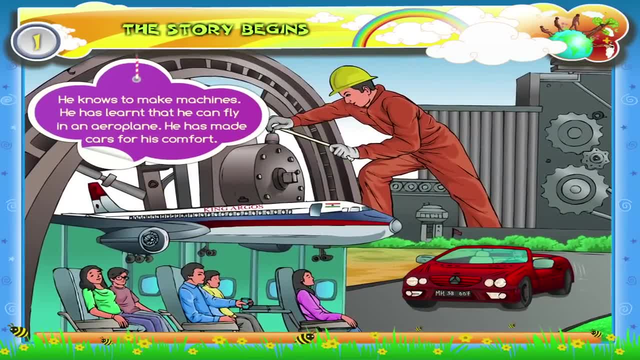 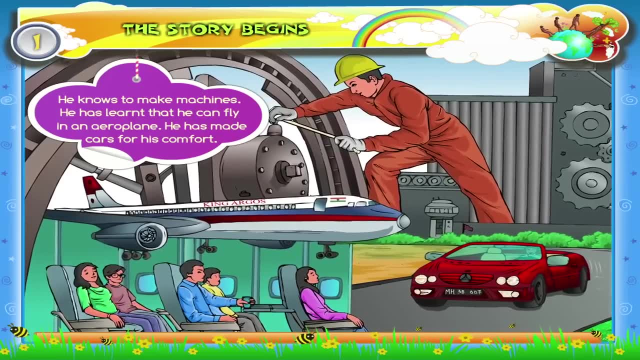 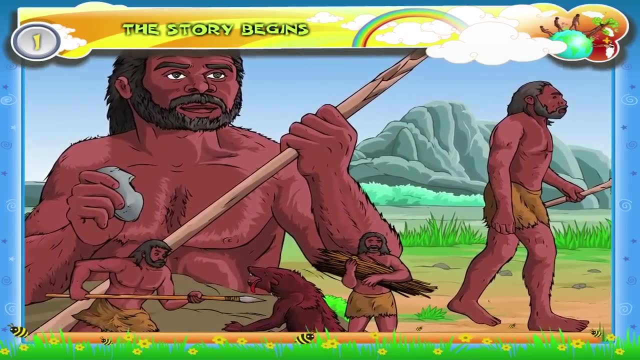 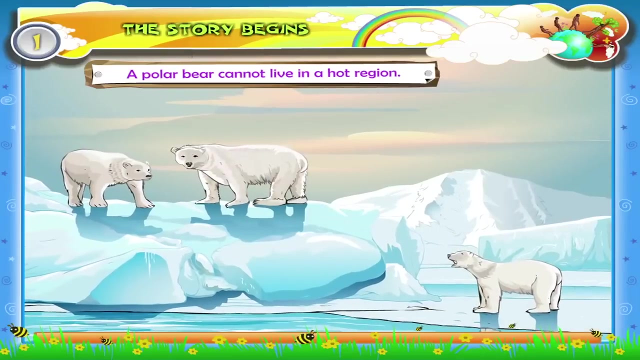 He knows to make machines. He has learnt that he can fly in an aeroplane. He has made cars for his comfort. Now isn't that amazing, Let's see. Let me tell you some more interesting facts about man. Just to give you an example, a polar bear cannot live in a hot region, but man can live. 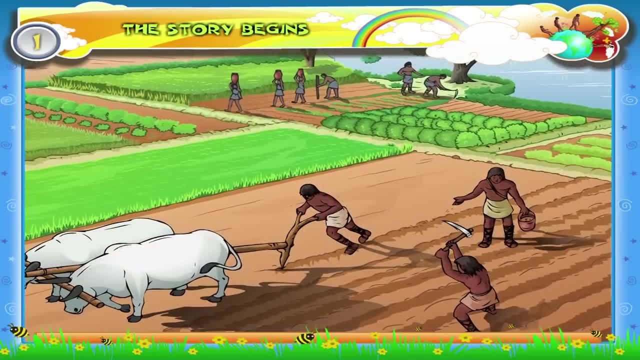 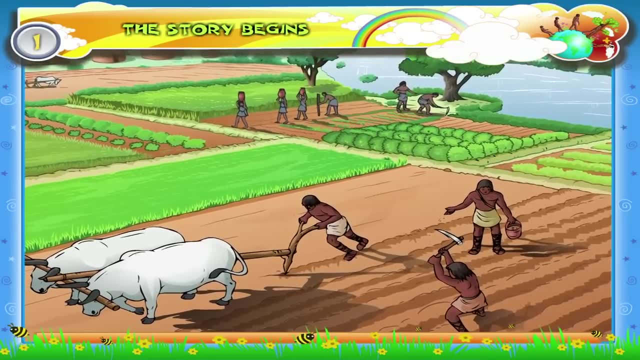 in a snowy region. This means that man can adapt himself to any environment. He can live anywhere on this earth. In cold regions, he wears woolen or woolen clothes. In cold regions, he wears woolen or woolen clothes. In cold regions, he wears woolen or woolen clothes.